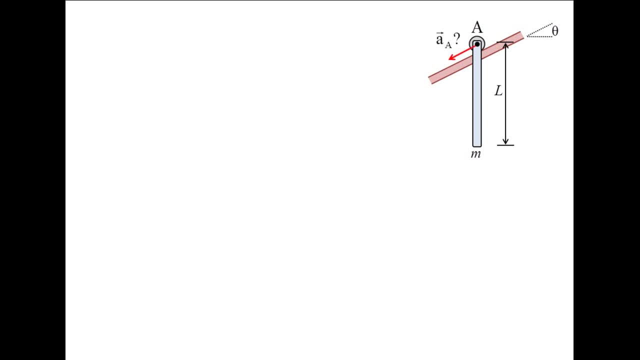 At this instant. what is the acceleration of point A and what is the angular acceleration of the rod alpha? Start by drawing a free body diagram of the rod, Identify your coordinate system and label the positive direction of your coordinates. In this case, a rectangular coordinate system is more convenient. 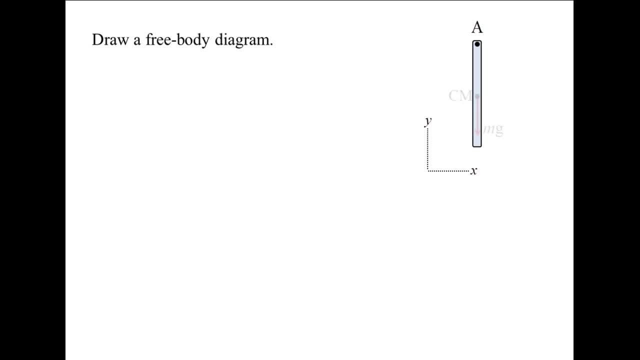 Draw the external forces acting on the rod. The weight acts at the center of mass and points downward. Its magnitude is the mass of the rod, m times the gravitational acceleration g. The normal force exerted by the surface on the roller n acts perpendicular to the surface at an angle theta relative to the vertical. 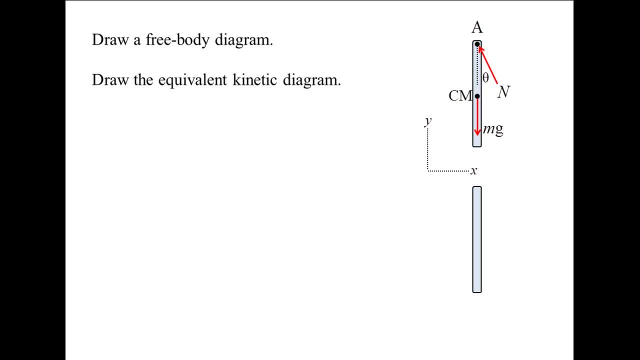 Next, draw the equivalent kinetic diagram, Select a positive direction for rotation, Draw the components of the acceleration of the center of mass and draw the moment about the center of mass, icm times alpha. We are ready to apply the three equations of motion. 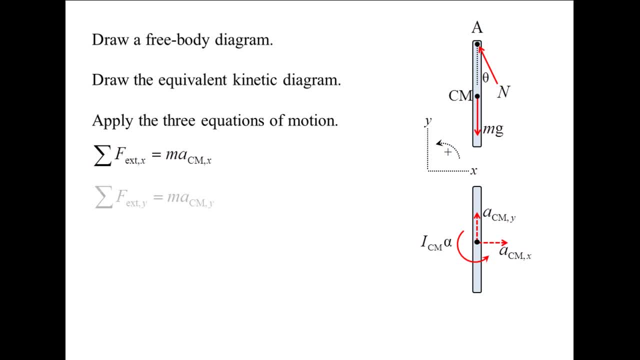 Newton's second law in the x direction, Newton's second law in the y direction and the moment equation about the center of mass For the x direction, the x component of the normal force points in the negative direction. The y component of the normal force points in the negative x direction. 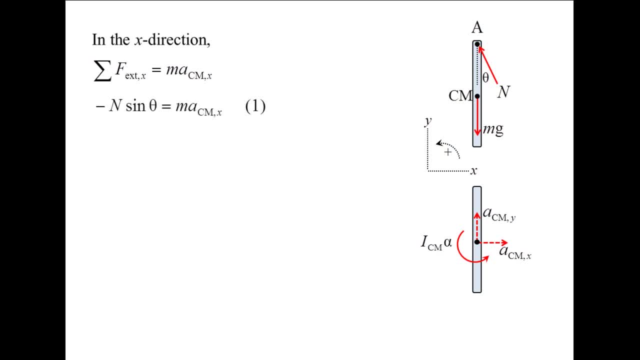 This is equation number one For the y direction. the y component of the normal force points in the positive y direction and the weight points in the negative y direction. This is equation number two For the moment equation, the moment of inertia- about the center of mass icm. 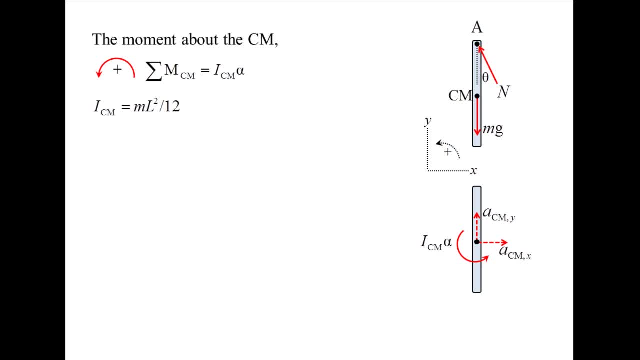 is the mass times the length squared divided by 12.. Next we determine the moment about the center of mass produced by the external forces. The normal force produces a positive moment and has a moment arm of 1 half l times. sine theta. The weight produces no moment because its moment arm is zero. 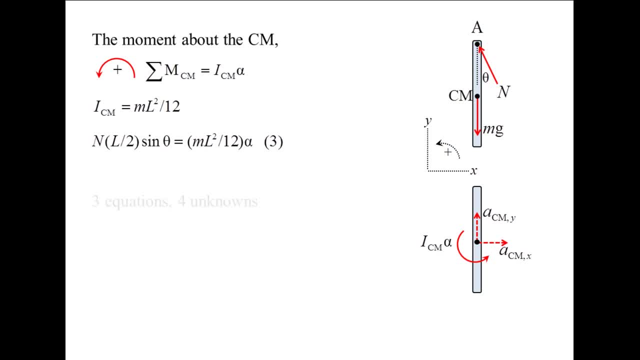 And now we have equation number three. We have used the three equations of motion but have four unknowns: N, alpha and the two components of the acceleration of the center of mass. Additionally, we want to find the acceleration of point A. 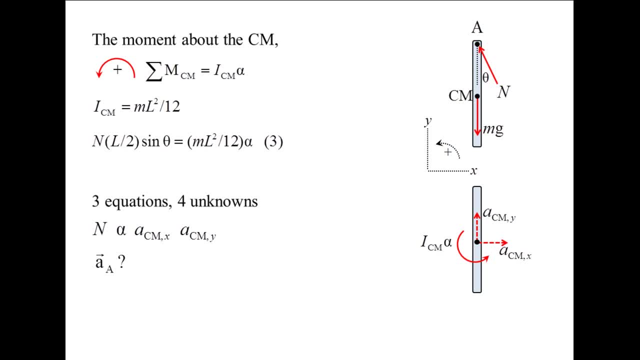 We can obtain two additional equations by examining the relative motion between point A and the center of mass. The acceleration of point A is equal to the acceleration of point A. is equal to the acceleration of point A The acceleration of the center of mass plus the acceleration of point A relative to the center of mass. 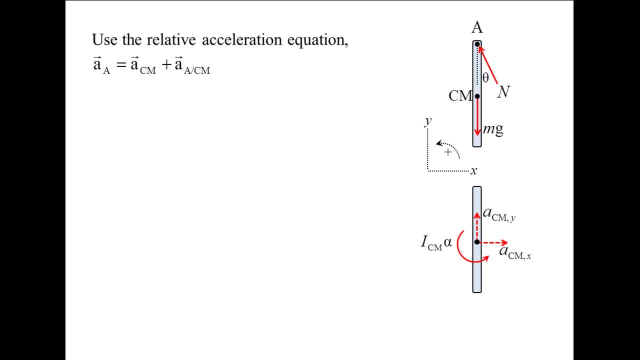 Although we do not know the magnitude of point A's acceleration, we do know point A must accelerate along the surface. The acceleration of point A is decomposed into its x and y components. The x component of the acceleration is the magnitude of acceleration times. cosine theta. 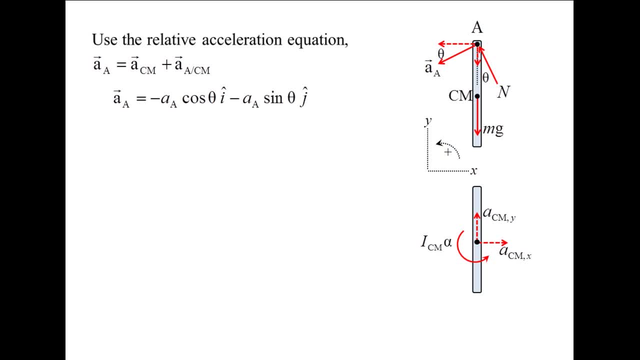 and points in the negative x direction. The y component of the acceleration is the magnitude of acceleration times sine theta and points in the negative y direction. ACM is decomposed into its x and y components. The relative acceleration term is decomposed into tangential and normal components. 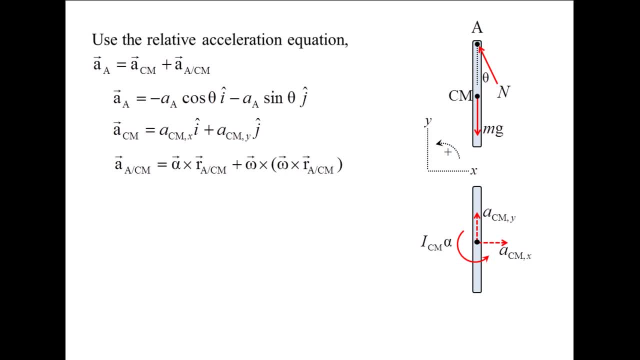 The tangential component is alpha cross- RACM, The position vector from the center of mass to point A. The normal component is the angular velocity of the rod: omega cross, the quantity omega cross- RACM. The angular velocity is zero at that instant, since the rod starts from rest. 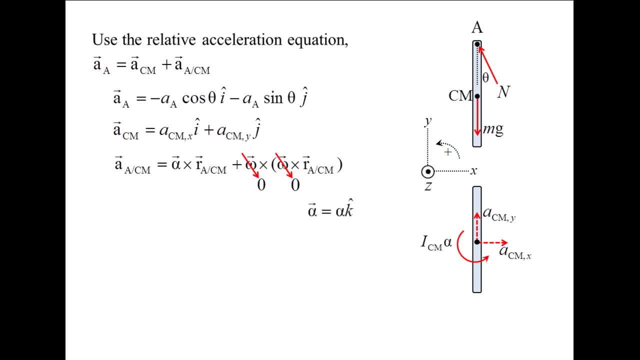 The angular acceleration vector has the magnitude of alpha and points in the z direction. RACM starts at the center of mass and terminates at point A. Point A is located one half L up from the center of mass. Take the cross product of alpha and RACM.